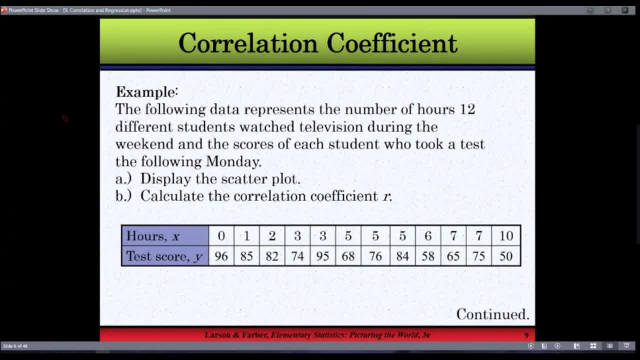 coefficient or So. this is the data. So we wanted to determine the correlation, or the relationship between the number of hours spent during the weekends and the score of the student during a test the following Monday. So we wanted to test whether, if you spent more or less number, 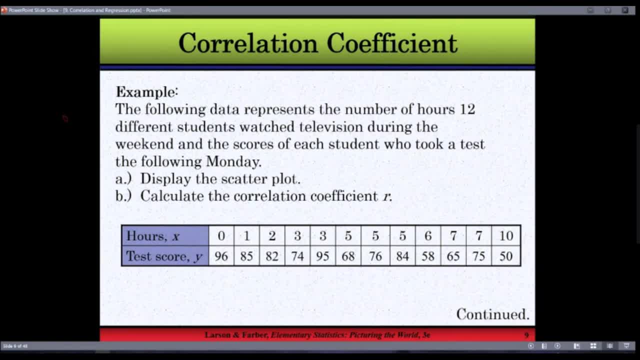 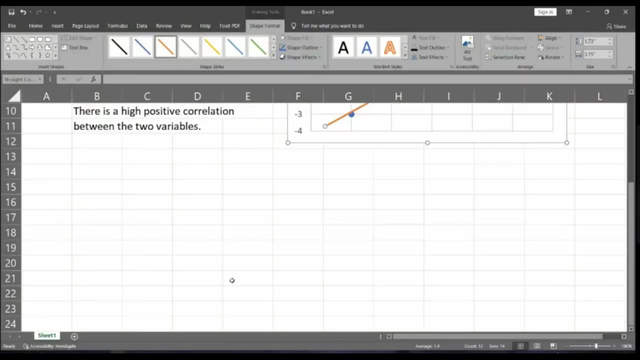 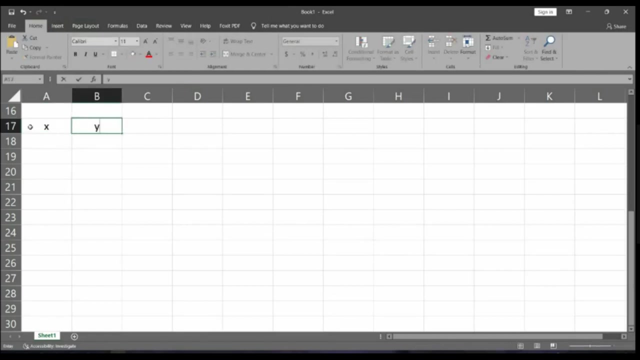 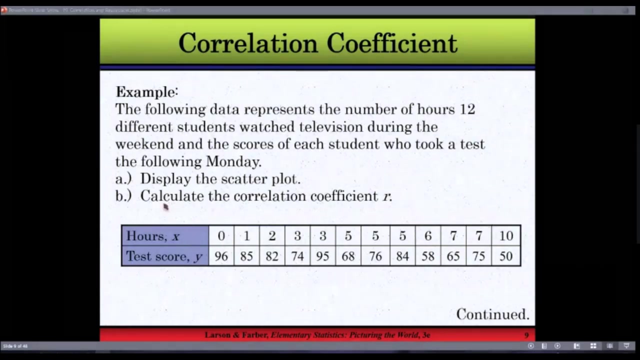 of hours watching television. is your score higher or lower in the test? That is what we are trying to define Using the correlation coefficient and the scatter plot diagram. So let's do that. I'll be copying this data in our Excel. So again, we have X and Y. So these are the number of hours Let me add. 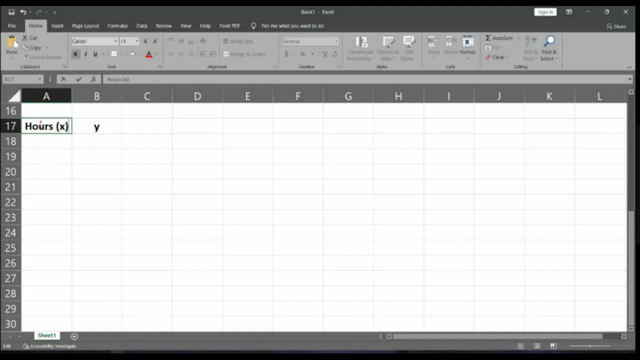 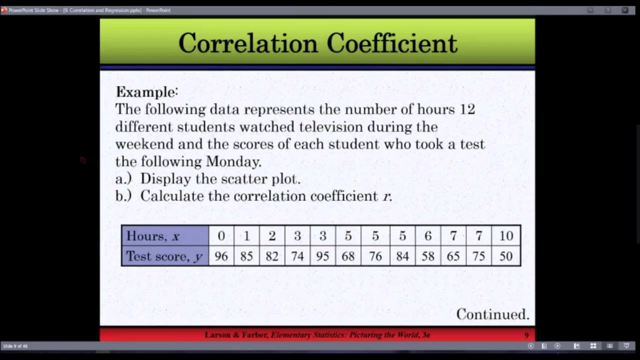 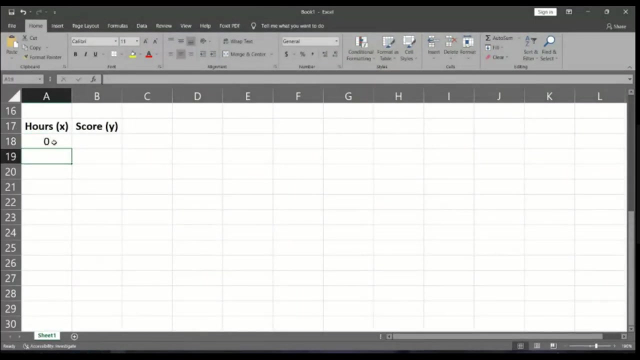 hours here And this is the scores, or the scores. So the first student did not watch during the weekend, So zero hour. Zero hour. Second student is one. You have two, three, three, five, five, five, six. 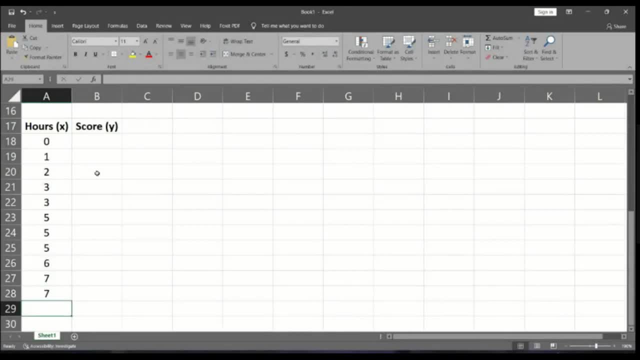 Two, three, five, six, seven, seven, ten, Six, seven, seven and 10.. Okay, Thank you. Do you have the copy? Yes, sir, Yes, Just saying this again. Please enumerate the Scores of these students. 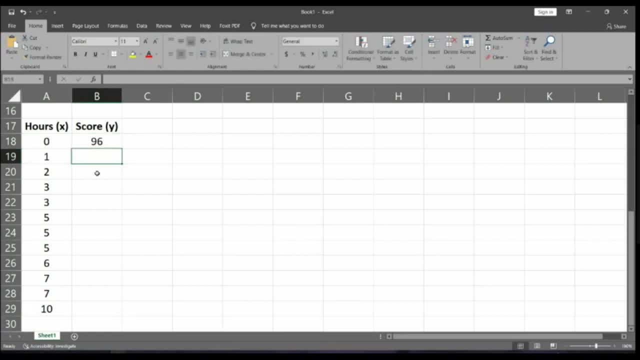 96.. 85., 82., 74. 95.. sixty-eight, seventy-six, eighty-four, fifty-eight, sixty-five, seventy-five, lastly, sir, fifty-five. thank you. okay, this is what we know about the 12 students, the number of hours they spent watching the television during weekends. 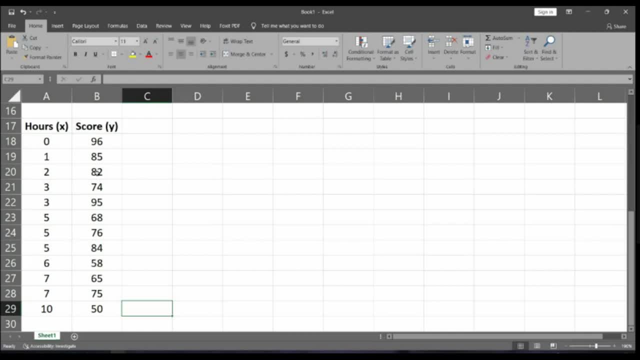 and their score the following Monday. so first is the scatterplot diagram. scatterplot diagram. so if you were using Excel again, I'll show you how to insert the scatterplot diagram using the Excel, so it'll be faster. so just go to the insert menu and look for the chart and 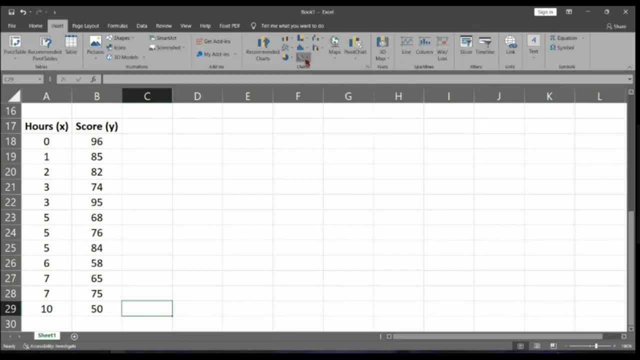 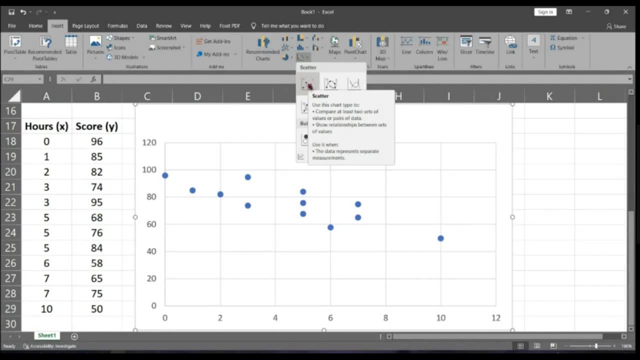 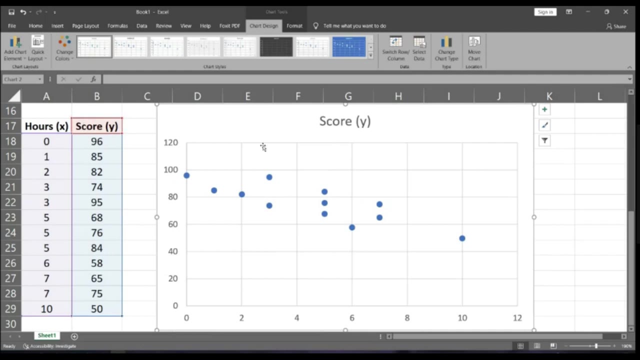 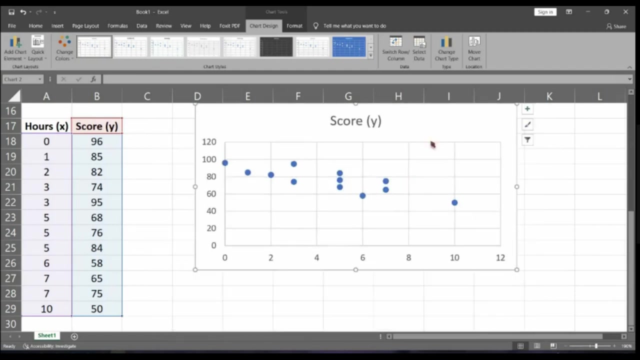 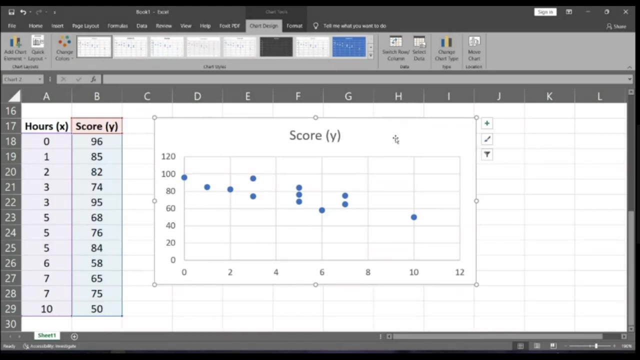 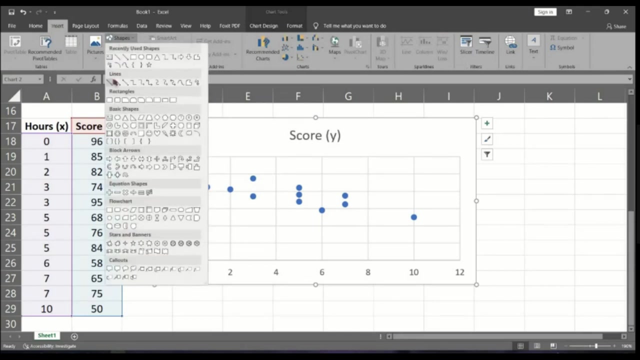 yeah, this is the logo for scatterplot diagram. choose the first example. I mean first, first choice. okay, so this is the scatterplot diagram. using this diagram, we can have an initial hypothesis hi about their relationship. so, as you can see, if we were to draw an imaginary straight line, 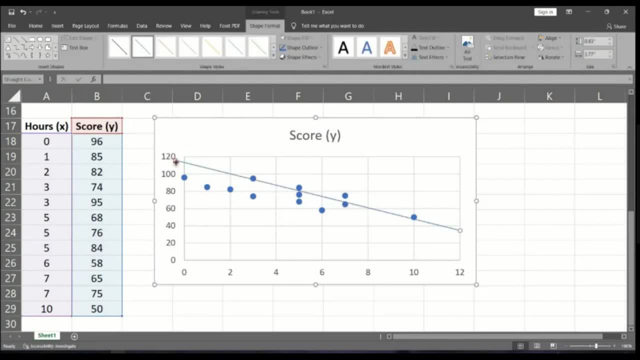 okay, this is the trend of the scatterplot diagram. now the points tend to follow this straight line and, as you can see, now the straight line is falling to the right, the slope of this line is negative. therefore, our initial hypothesis is that the two variables are correlated or positively correlated. okay, two variables are positively. 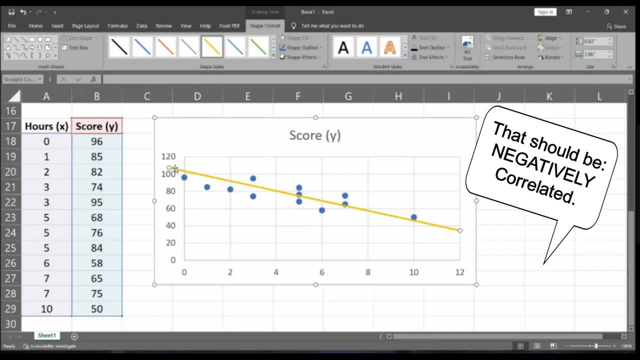 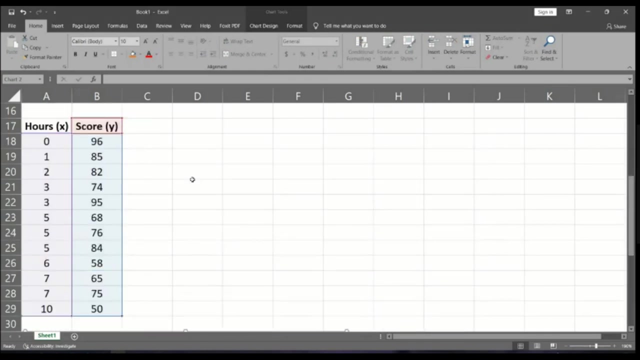 correlated. so the question is, how much? how much they are correlated, how much, how strong is the correlation between them? and that question will be answered after we computed for their coefficient, the correlation coefficient. So that is the second one, Set aside first the scatter plot diagram. 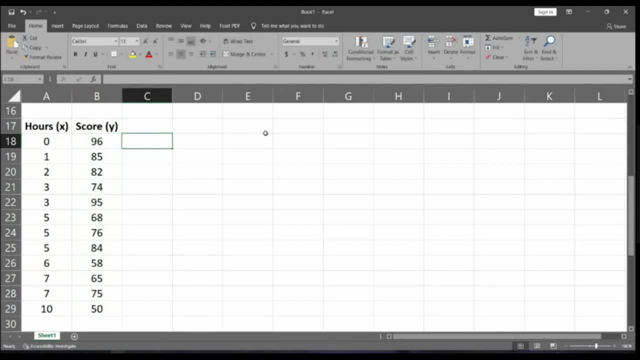 And let's proceed to the coefficient. Okay, So we need to add columns for their product: x times y. Okay, Another column for the square of the first variable and the square of the second variable, And so just multiply them: 0 times 96,, 1 times 85,, 2 times 82.. You may use your calculator. 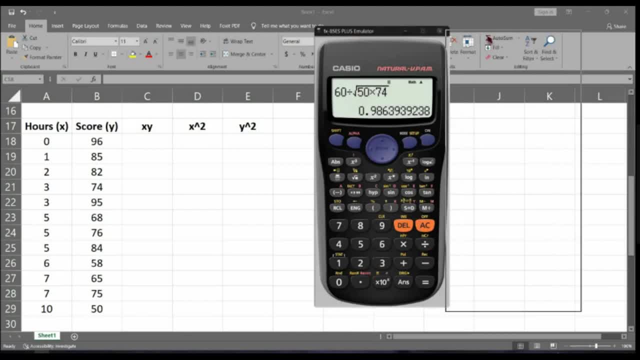 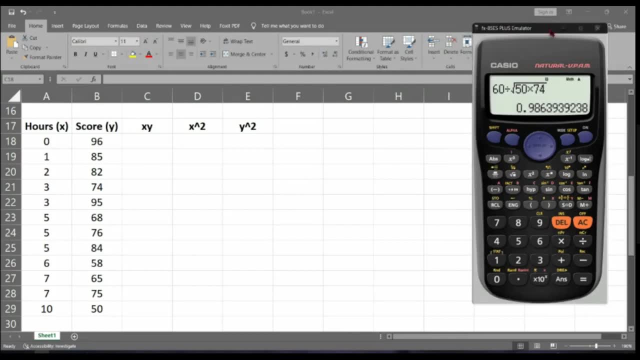 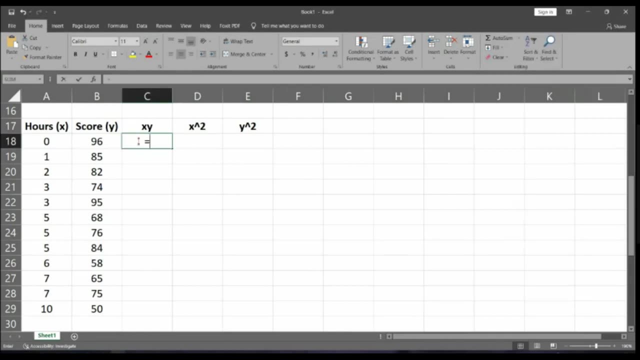 You may do it manually, But if you were to do so, it will be longer The time that you will consume. If you were to use Excel, it's very easy. Just use the feature Type equal sign. This will prompt you to include the formula. 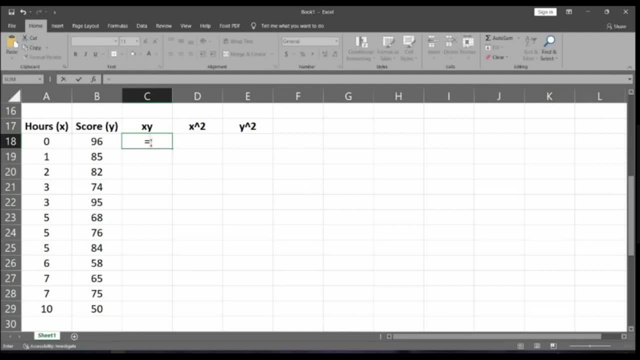 The formula that you wanted to do. Okay, Given these values. So I would like to multiply this, The cell, The data in this cell, with the data in the cell. Okay, Take note. The symbol for multiplication in Excel is the asterisk sign or the star sign. 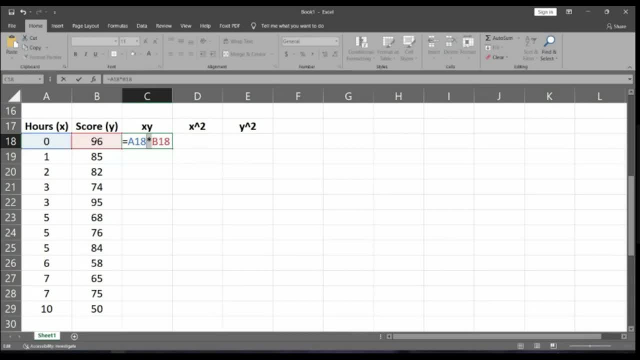 So take note of that Meaning. I were to multiply 0 and 96 here, Which is equivalent to 0.. Okay, And do it again: 1.. Times 85.. Okay, Or you may just click this cell and toggle this little square below the cell. 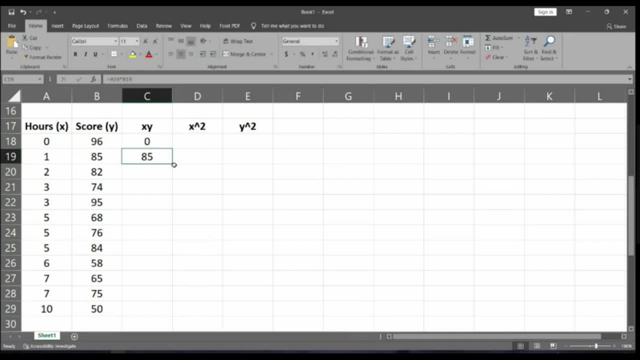 And if your cursor changed into the cross, Drag the square. Just click Right-click and then drag this up to the last pair of X and Y, and then that's it. you'll have the product of X and Y. okay, as simple as that. next, next column: we need to square, you need to square the X. 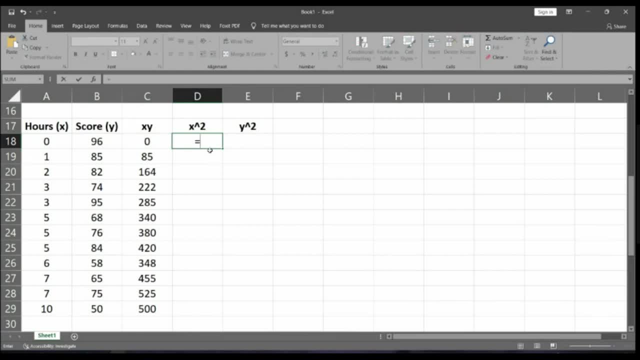 variable. so, using the formula again square, you may use the symbol. I just look for the symbols, some keyboards, you know that is zero square, I'm sorry, square. hey, you cannot find that symbol? then you may just multiply the same cell by one times one. a one times one, that is good as one squared. it's up to you know. 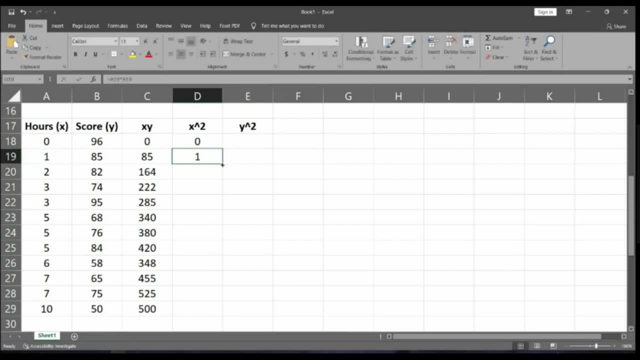 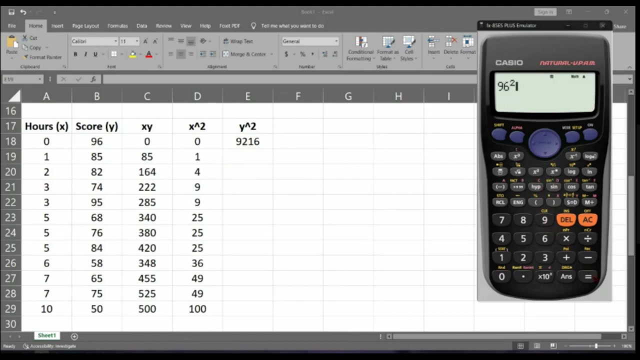 it's up to you which, which one you are moving to most comfortable with, and then drag, that's it okay. and then for Y, this is Y squared. I would like to use squared that at the six times 96 if you want to confirm that. you may use your calculator and see if this confirms your Excel. 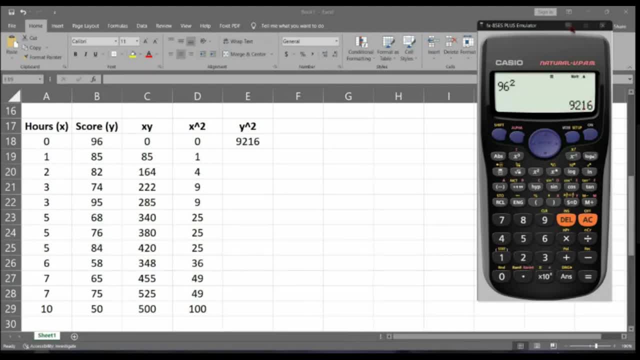 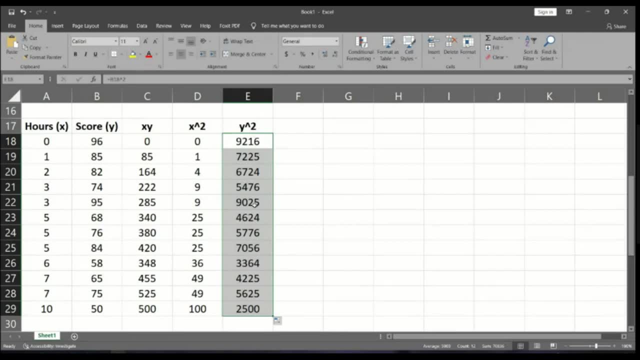 which is, through the man, nine thousand two hundred sixteen. so you may drag again the formula to be copied to the rest of the cell. and that's it. we now have completed the table. hi, the table. and the next next would be the prod, i mean the sum, the sum of all the columns. summation of x. summation of y. summation of x- y. 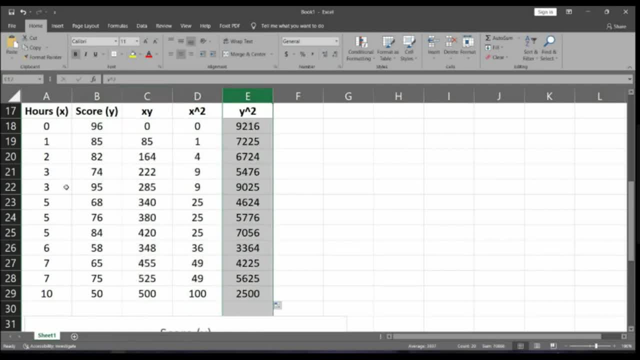 summation of x squared and summation of y squared. so manually. but then you can add that one by one, but be sure to be sure to input the right values. no, okay, the tendency it is my values, so your solutions will be messed up so that but accurate when using. 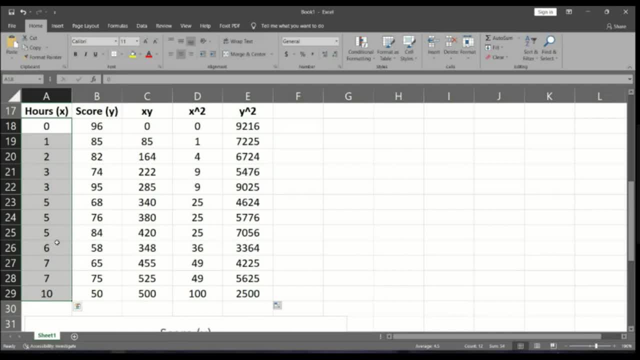 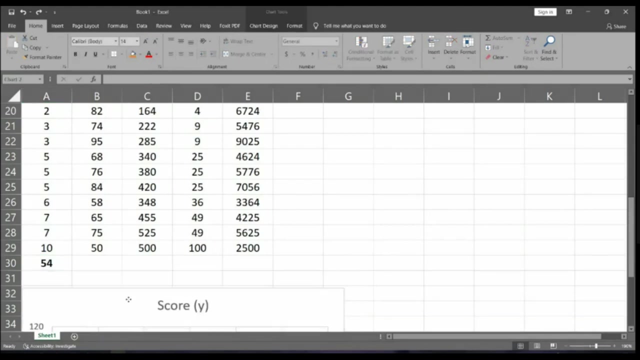 your calculators manually. but for excel, just look for the auto sum feature. this will auto add or total higher the the highlighted cells. okay, so click on that and you now have 54.. that's it. this time we'll drag. we'll drag, oops, vertically, or i mean horizontally. 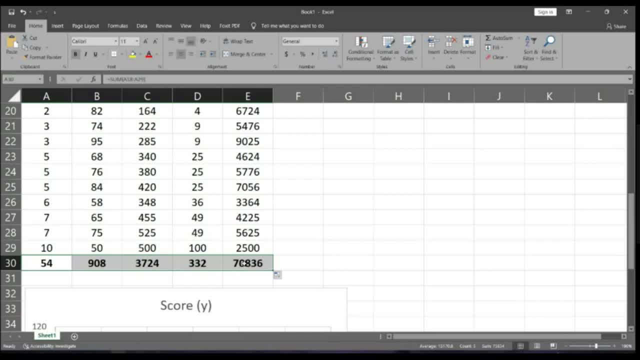 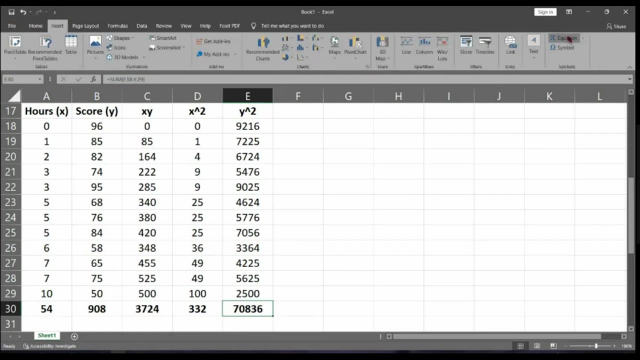 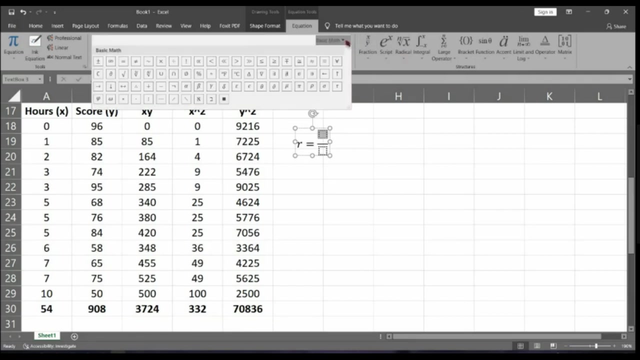 and the formula will be copied. you now have these values: 54 908 3724, three, three, two, seven thousand eight hundred thirty six, and using these values, we may now, uh, use the formula of pearson r. okay, this is r, so remember the formula. do you remember the formula? i won't ask you to. 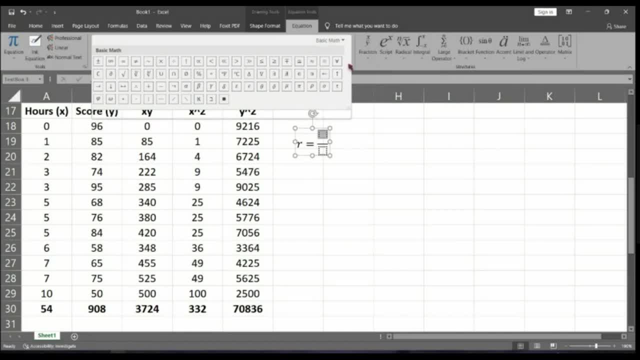 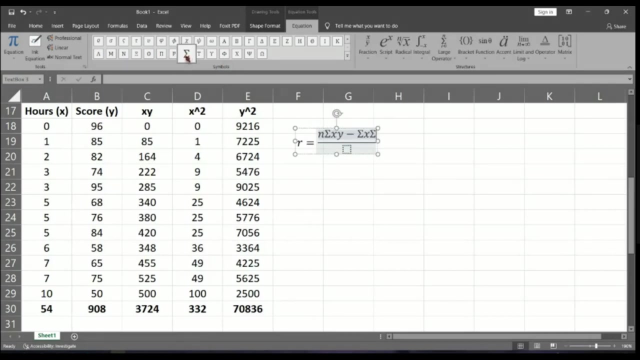 memorize the formula. no, you may just, uh, you may just copy the formula reference in a index card or clean paper or whatever. but i'm a radical formula jet. so we have n times summation of x, y minus summation of x times summation of y, all over square root. 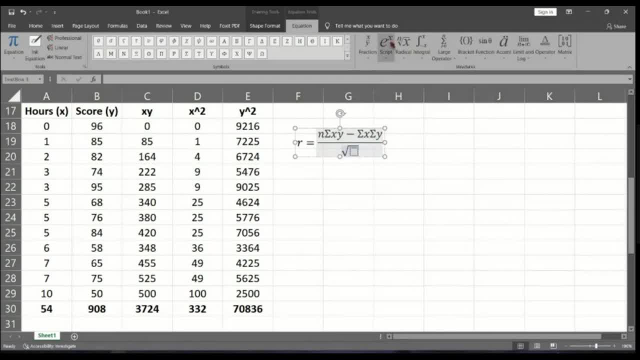 so i give another one down. okay, i'm going to add here this, because i know we're in this left over section, so actually there were two square roots there now. so and we have n times summation of x squared minus quantity. don't forget the quantity. summation of x. 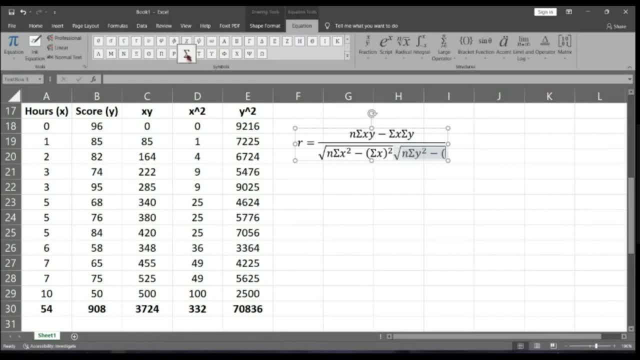 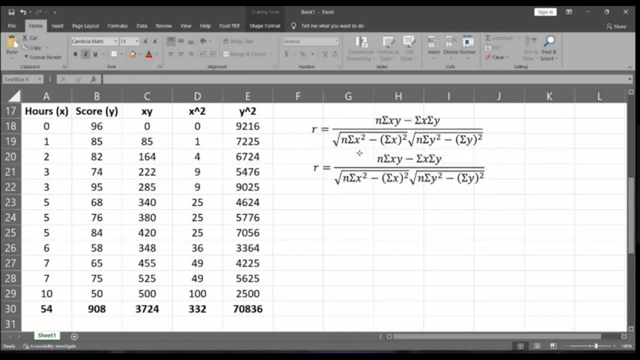 minus the quantity summation of Y, quantity squared, and this is your formula. this is the formula, and we may now substitute the values. what is our n? how many students were involved? how many pairs of data we have, guys? how many pairs of data we have? hi, we have 12. 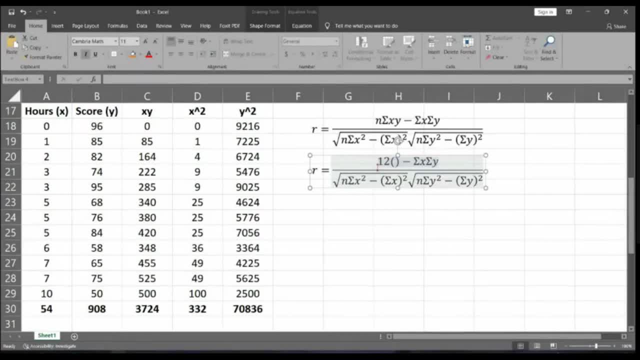 summation of XY, you have 3724. summation of X is 54, summation of Y is 908, and then we have the same n. summation of x squared is 3, 3, 2, and then summation of x is 54. well, 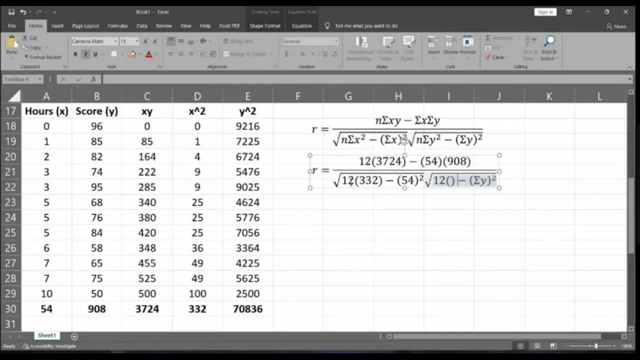 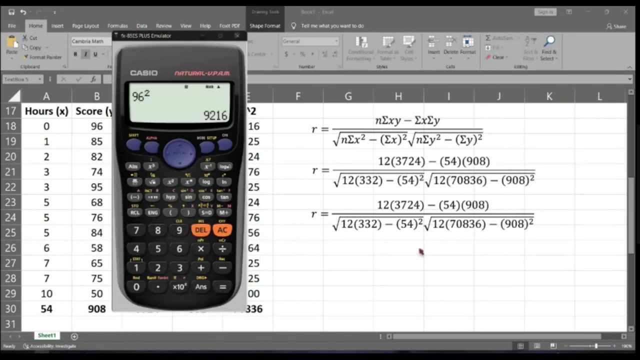 times summation of y squared, this is a large value, no, seventy thousand eight hundred thirty six minus summation of y. and then that's it. and let us simplify each part, the numerator and the denominator. let's start with the numerator, using our calculator, so just input everything: twelve thousand by. 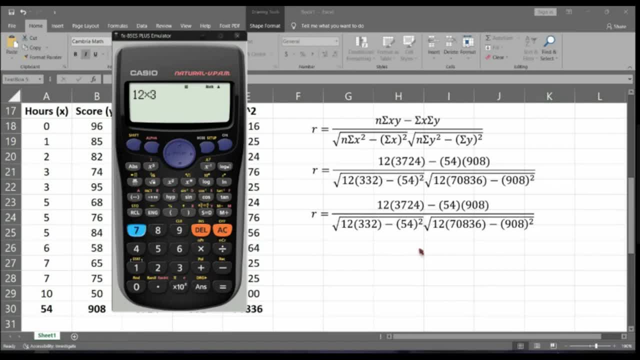 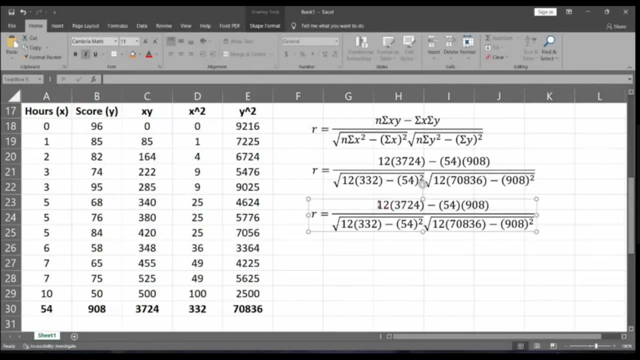 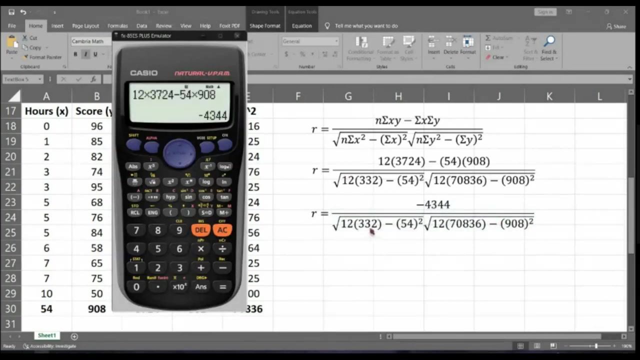 element: twelve times three thousand seven hundred twenty four minus fifty. four times nine, oh eight, and then that's it. the salt is negative four, three, four, four. negative four, three, four, four. I done with the numerator, the first radical. we have 12 times three, three, two minus fifty four squared. 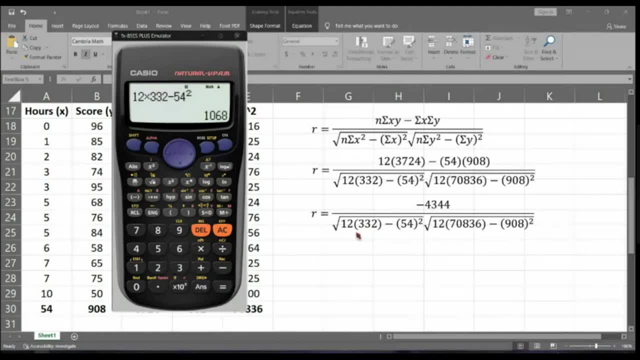 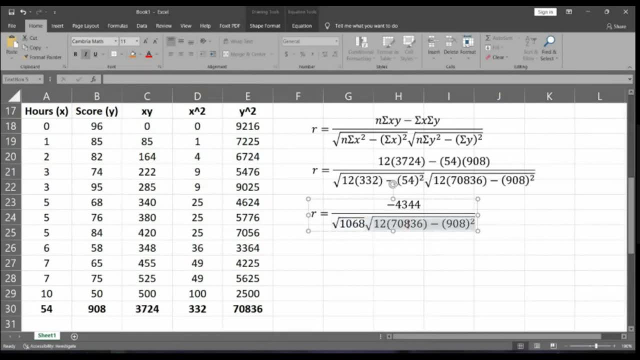 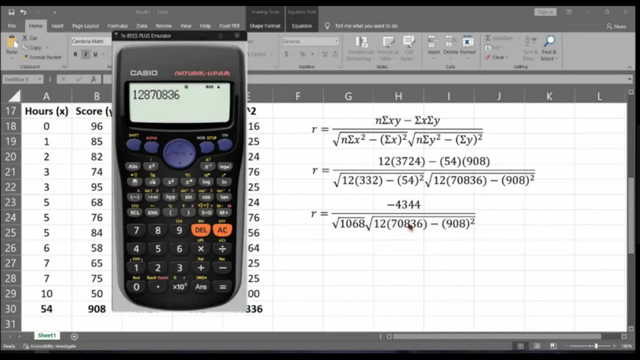 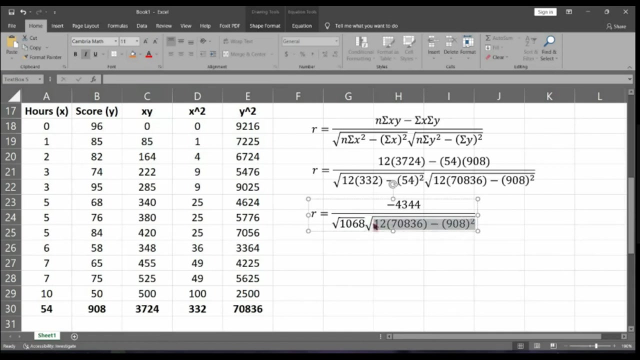 fifty four squared, it's 1068, and the other radical. you have 12 times seventy thousand eight hundred forty six- which where is the duplication sign? and 12 times seventy thousand eight hundred forty six minus nine hundred eight squared, you have two five five six eight. two five five six eight, and then that's it. okay, we may now. 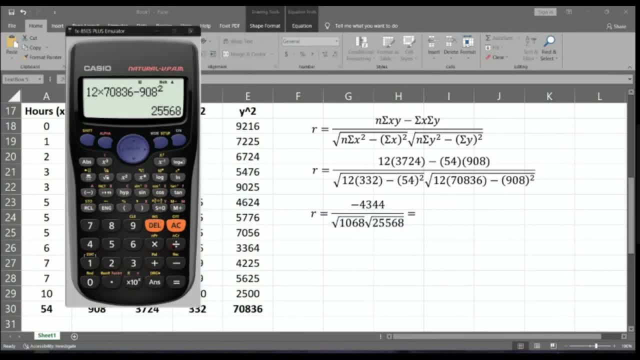 include everything in our calculator. you have negative four, three, four, four, divided by square root of 1068 times two, five, five, six, eight. again I buy properties of radicals same since this. two radicals have the same index, I, but I also like square root. we may just multiply their radicands by 1068 and two, five, five, six. 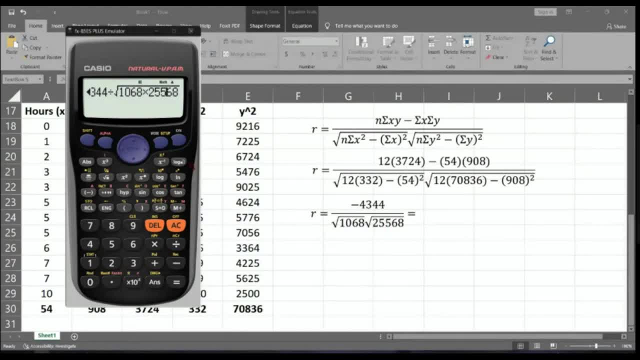 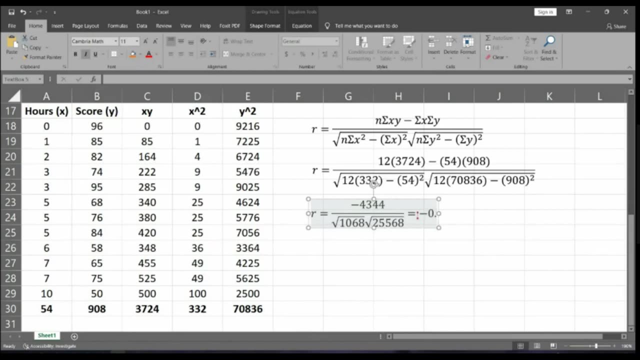 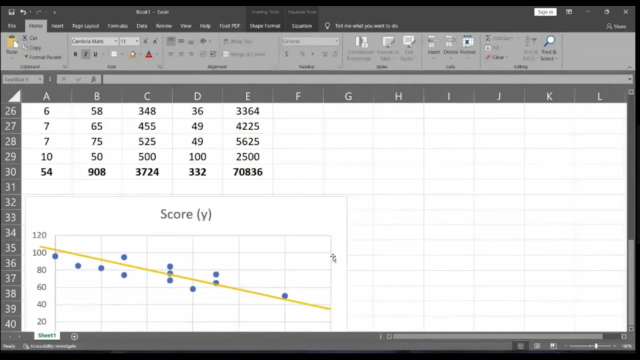 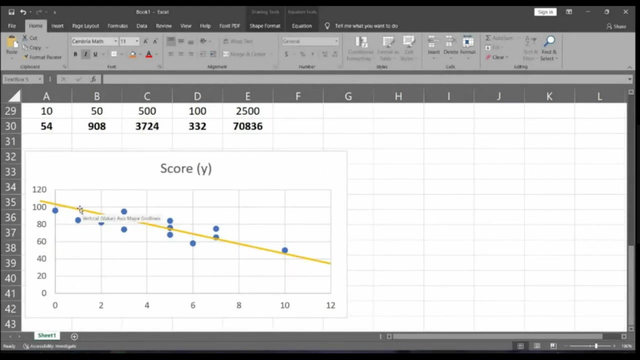 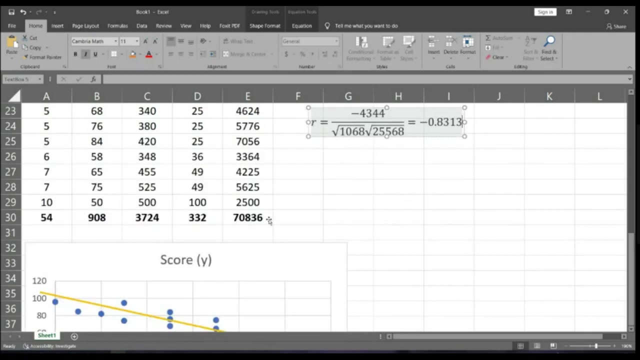 eight and whatever the value here will be, our coefficient equals negative zero point eight three one three. negative zero point eight three one three. so this is your coefficient. this confirms our scatter plot diagram about this is negative. okay, this is negative. the slope of this line is negative and, at the same time, very evident because the coefficient is very. 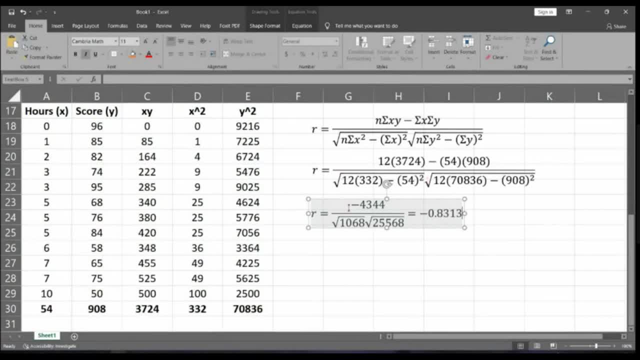 close to negative one. okay, so we may now go interpret this result interpretation: there is a high negative I correlation between the two variables, but this time I would like you to be very specific. now, what are the two variables? there is a high negative correlation between the number. 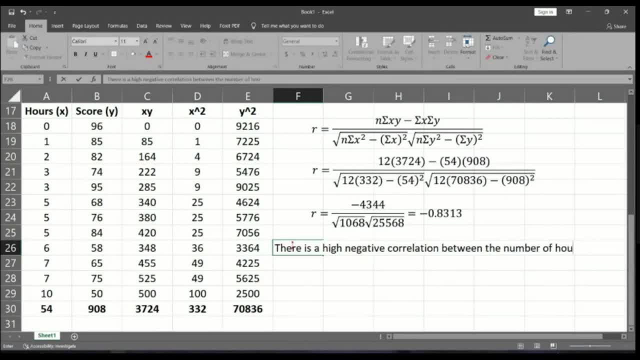 of hours, the number of hours spent watching television during weekends, and the other variable is, and the other variable the score course of the score scores of the students- students in a mess and his course of the students in a score scores of the students- students in a test during any test duringなんか. gresae possible are very commonbrand rare in India but never at all is cause a common grad in the world. ok, testing from two students in a number, three hundred and five years gone to another one, three here. p here is also common sense to be a tusser who burn help management. technology'm just see, but it soundswise the unit room right, a popup little hang on jams in here. someone else wanted to let you say hey, Rosal, previously dip, so please shut off here's this. but okay, we have also take some other variables, the number of the camp. so we want to know who is correct. what will we give?